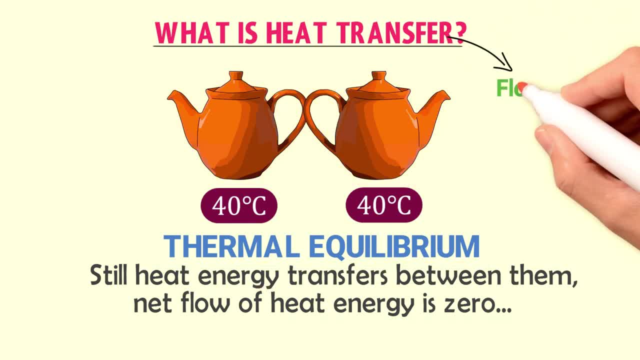 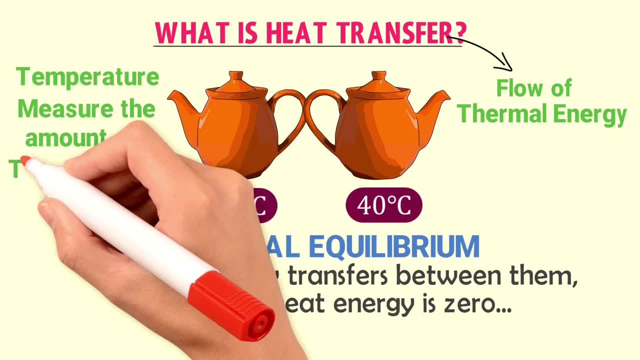 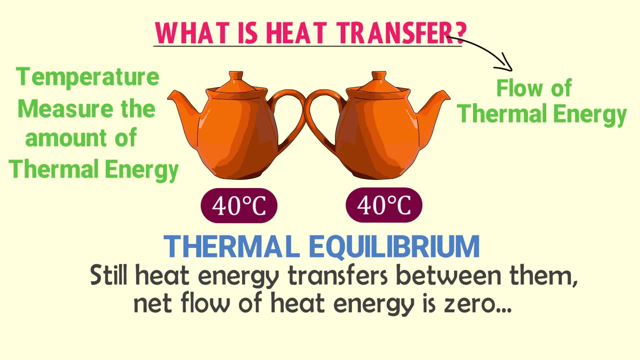 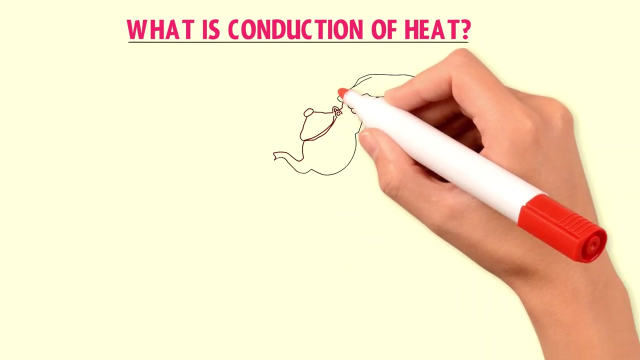 equilibrium. Therefore, remember that heat transfer is the flow of thermal energy, from thermal energy, heat energy between two objects, While temperature only measures the amount of heat energy possessed by an object. Now let me teach you the concept of conduction, or what is conduction of heat. Let's consider a very hot object and you 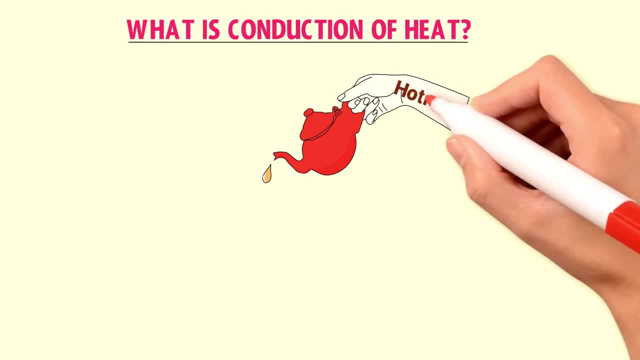 suddenly touch it, Your hand feel the hotness or your hand may be burn. Why your hand feel hotness? The answer is that some of the thermal or heat energy of this object transfer to your hand. As a result, your hand give hotness. Now let's consider another case. If you keep away your hand from this hot, 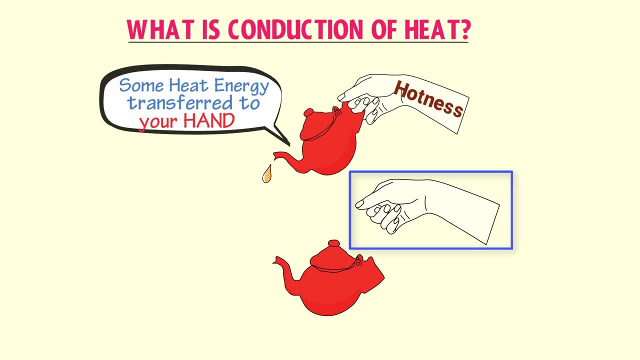 object. does you feel the hotness of this hot object? the answer is no, Because in this case your hand touched the object hot object. are there is contact between your hand and this object, while in this case your hand is away from this hot object. are there is no contact between? 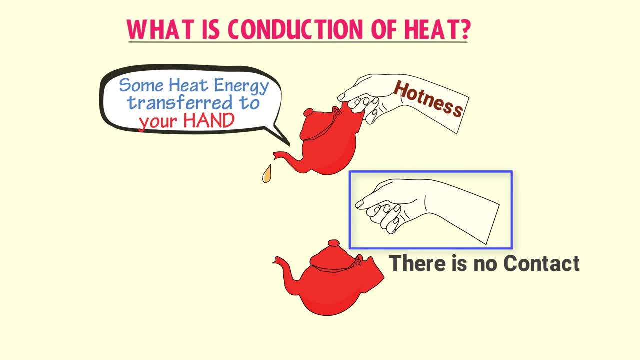 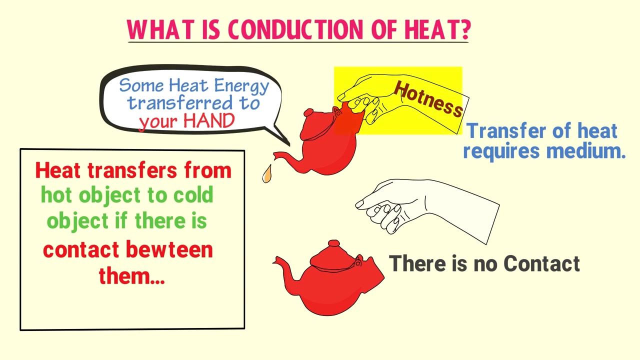 your hand and this hot object. so from these two cases we learn that heat only transfer from hot object to cold object if there is contact between them. are in physics we say that flow of heat, our transfer of heat requires medium. here your hand is cold and when you touch this hot object your hand provides. 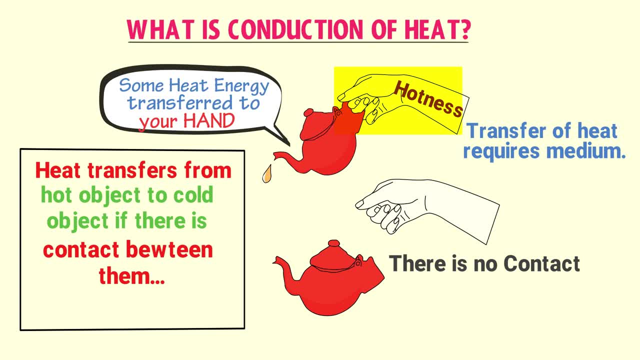 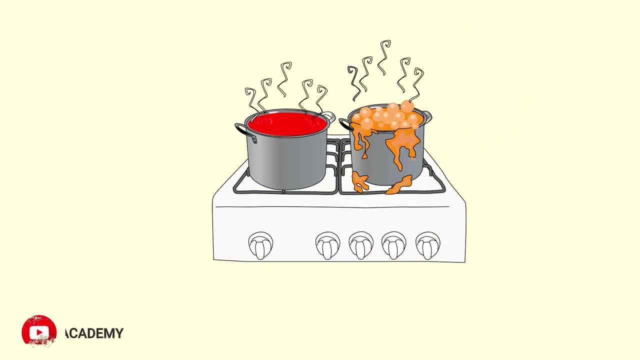 medium to heat energy present in this hot object and it travels towards your hand. as a result, you feel the hotness. let me give you another example. for instance, you are cooking some sort of food. You always place the frying pan or pot exactly above the fire or flames. 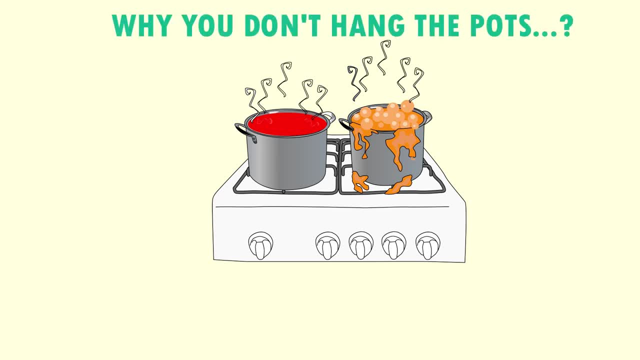 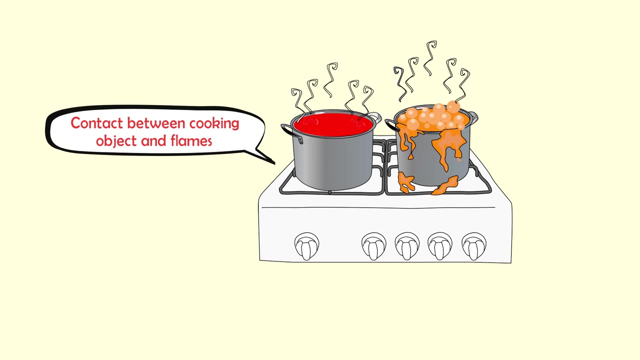 Why you do not hang or place the pan or pot away from the fire. So you aren't doing so. You always place the object straight above the fire. It is because there will be contact between your cooking object and flames. Thus this contact will provide medium to heat energy. 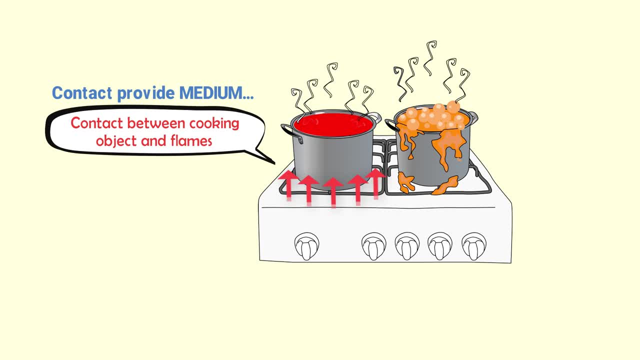 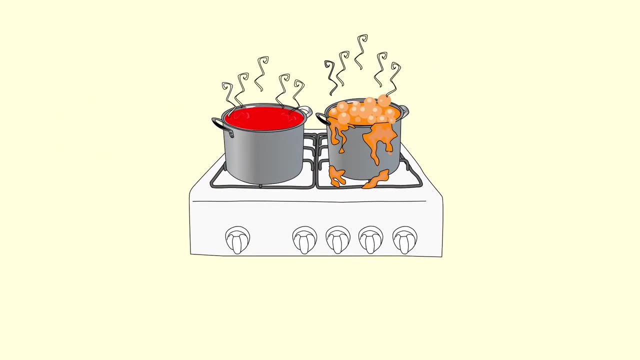 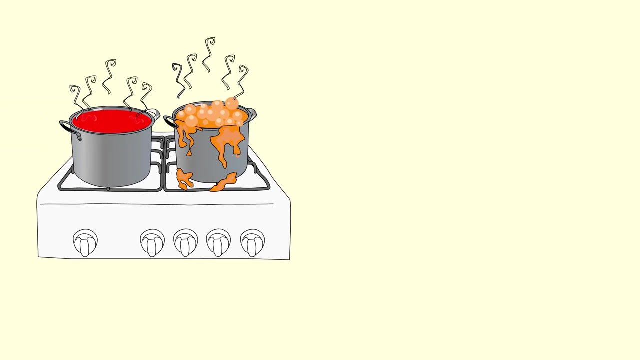 Due to which heat energy or thermal energy of the flames would transfer to your cooking object, And food will be cooked by this way. Now let me give you a deep dive so that you could learn the scientific explanation behind this phenomena of heat transfer. We know that cooking objects are made up of metals. 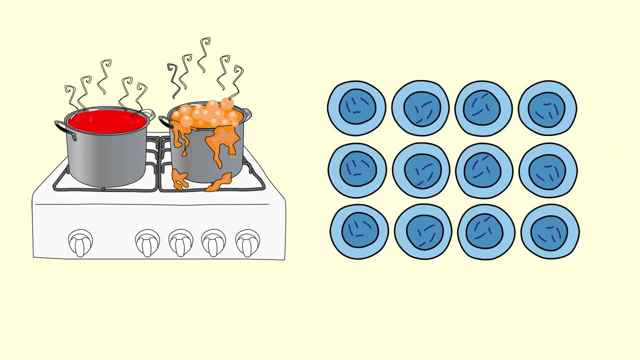 The atoms of metals are closely packed together And a uniform three-dimensional pattern. When you place this cooking object or pot made up of atoms on fire, The atoms of this object get heat energy and start vibrating vigorously. Now this atom will transfer heat energy to this atom. 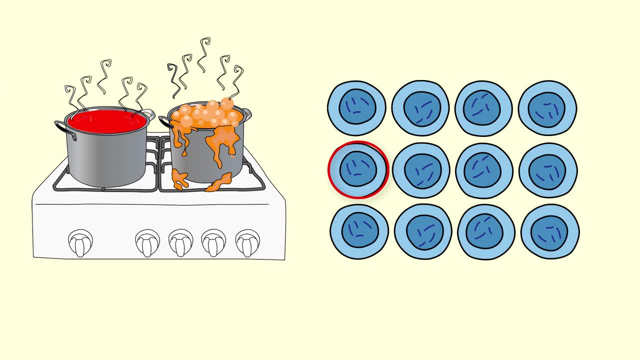 While this atom will transfer heat energy to this atom. Hence, by this process, The heat energy will start flowing among the atoms and your food will be cooked. Thus, this flow of heat energy from fire towards the cooking pot, without transferring atoms or metal, is known as a conduction, or conduction of heat. 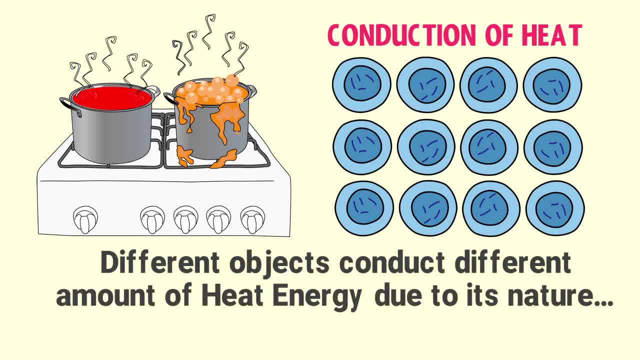 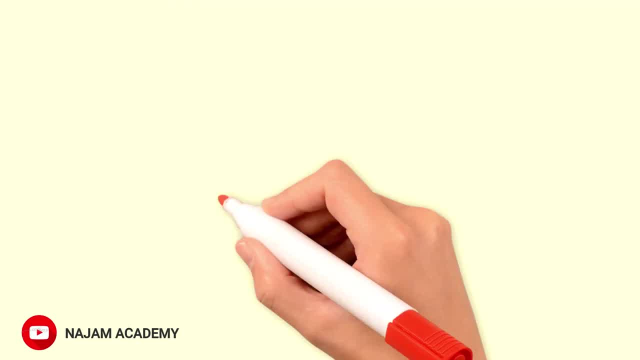 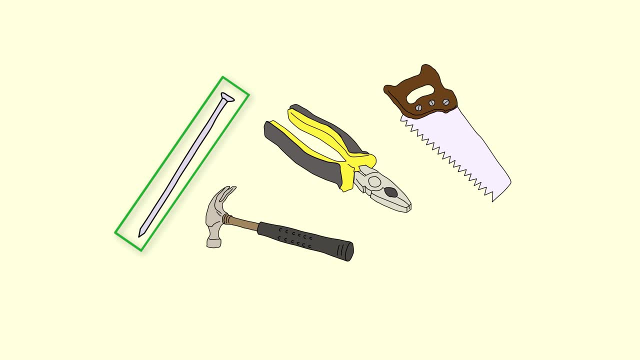 Remember that different objects conduct different amount of heat energy Due to their nature of material they are made up. Let's consider These objects. this object is made up of iron, so it's thermal conductivity would be large, While the handle of this object is made up of plastic or wood. 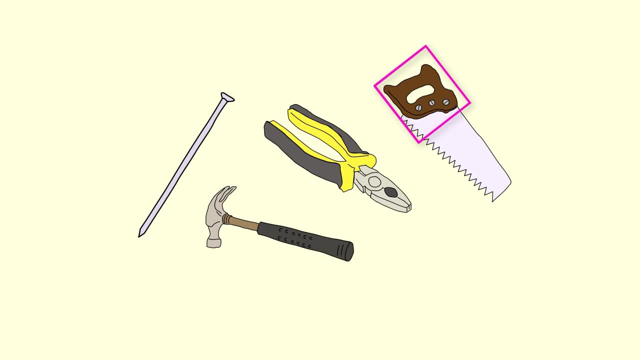 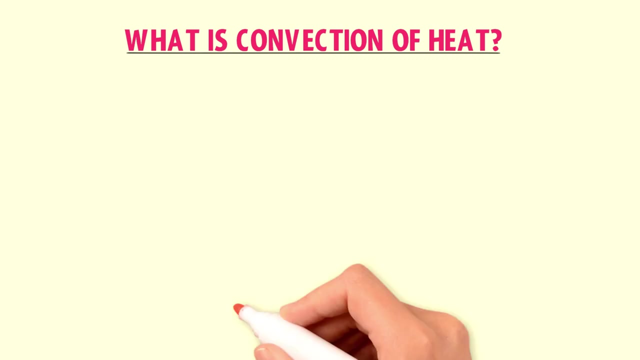 While plastic and wood are insulators, Hence thermal conductivity or current conduction would be minimum. and them? Now let me clear your concept about what is convection of heat or conduction of heat heat. Let's consider, if you place your hand slightly above the fire you feel 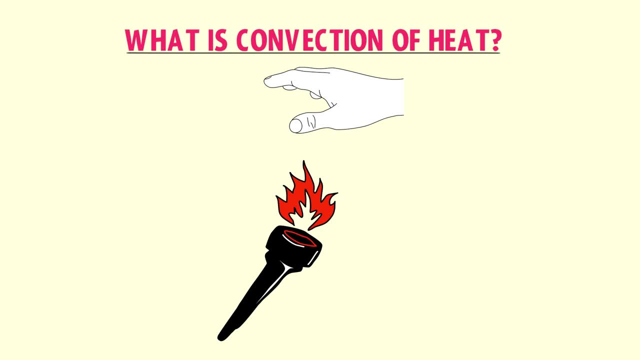 the hotness of fire. In the previous slides we learned that heat energy was only flowing when there was contact between hot object and cold object. but here, in this example, your hand doesn't touch the fire means there is no contact or no medium. Well, the scientific answer is very simple. Do you know the word? 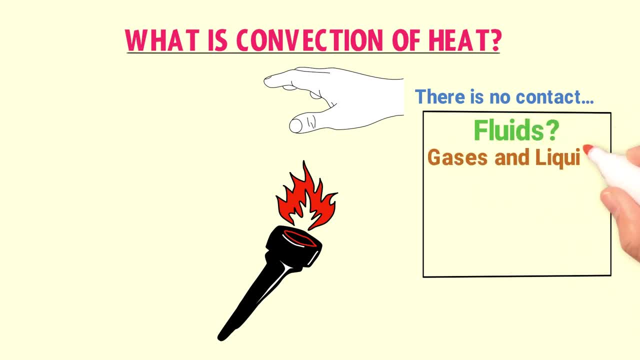 fluids. The word fluids means gases and liquids. We also know that gases and liquids are in random motion. Other molecules of gases and liquids possesses kinetic energy. Now here is the important point: The kinetic energy of gas and liquid molecules is the energy of gases and liquids. 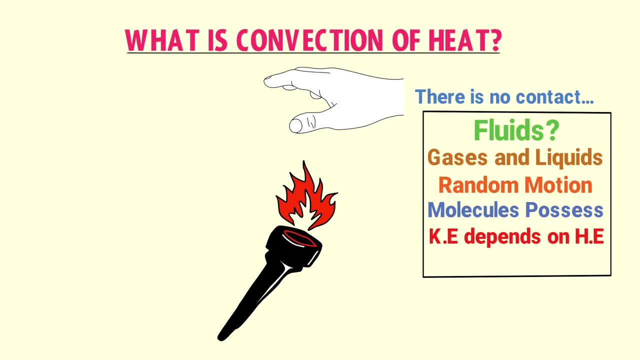 Depend upon heat energy or temperature. Keep this point in your memory. and let me now explain this case. We know that there is air above the fire or flames. Hence the gas molecule absorb heat energy from the fire. As a result, the kinetic energy. 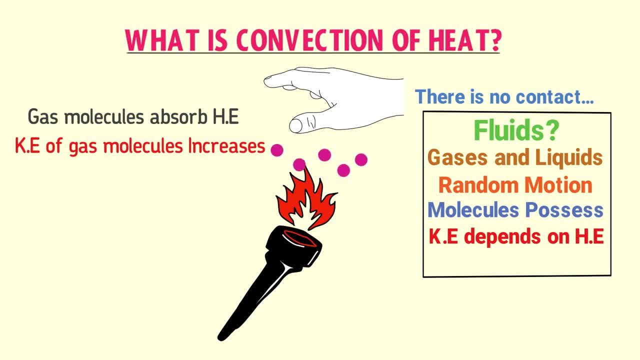 of these molecules increase. Hence they rise up and hits your hand. thus your hand is blocked. Now remember that the kinetic energy of this liquid molecule is also hand being cold. absorb the heat energy from these gas molecules and you feel hotness. Therefore, remember that in this case, gas molecules are fluids, are transferring heat energy from the fire. 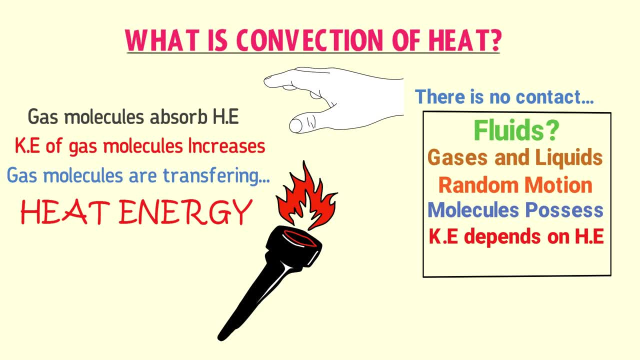 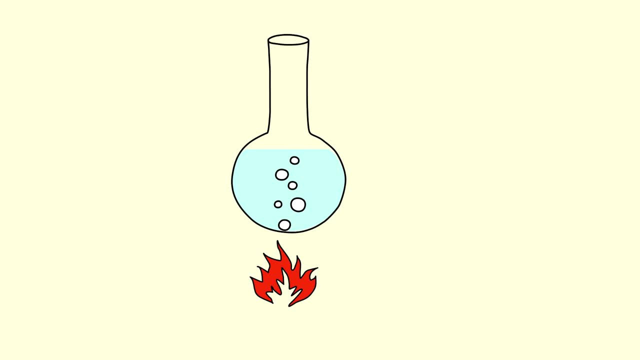 to your hand. The another example of convection is boiling of water. Let's consider that we place an object filled with water on fire. Now there is contact between fire and this conical flask. So by the process of conduction heat energy from the fire would transfer to the water. Now water 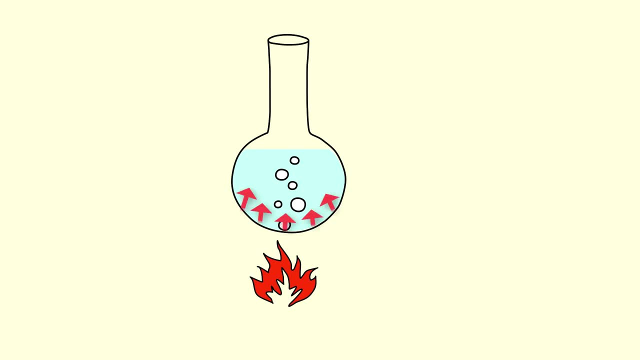 being fluids, its molecule will absorb heat energy from the flask and will rise up. Here let me ask you a question: Why these molecules of water rise up After getting heat energy. The answer is that they become less denser, and let me repeat this. 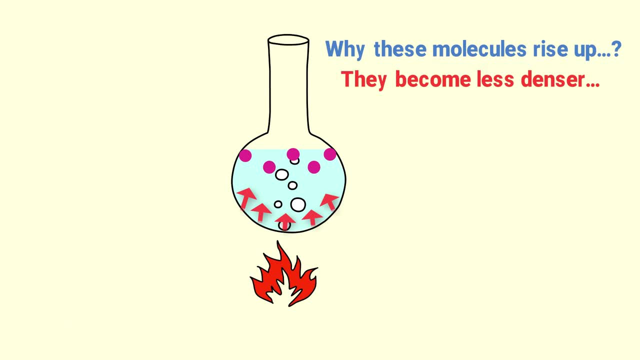 important point. The water molecule rise up because they become less denser, while the same surrounding molecules of the water are more denser. Thus, due to this, they rise up. Now the denser molecules at the top falls down bottom. After absorbing heat energy, these molecules will also rise up. Thus the less 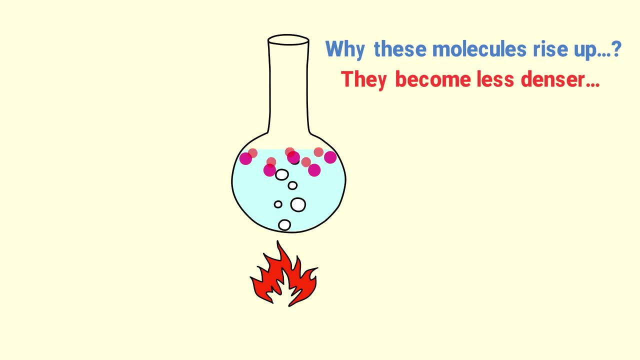 denser molecules of water rise up and the more denser molecules fall down. This process would be continued until all the molecules of water get heat energy. A time will reach that the kinetic energy of these molecules will be maximum and a change of state will. 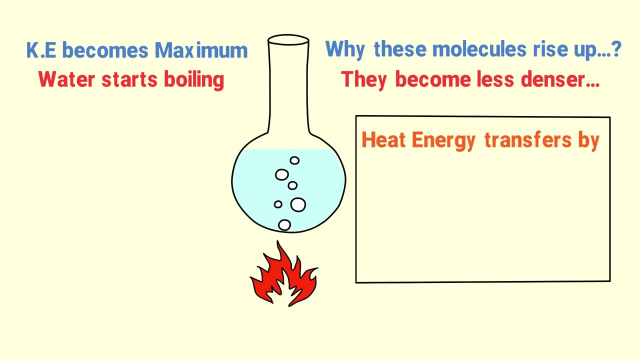 occur, Water will start boiling Here. heat energy transfer in water by the motion of molecules from the bottom to the top. This motion is called bulk motion of fluids, Hence the transfer of heat energy due to bulk motion of fluids from one place to another place. 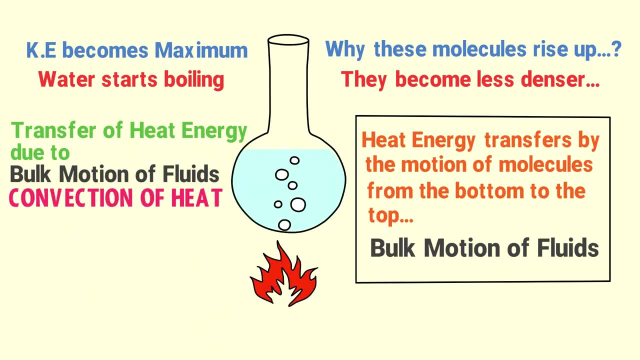 is called convection of heat. At last, let me teach you that: 1. What is convection of heat? 2. What is convection of heat? 3. What is convection of heat? 4. What is radiation of heat? 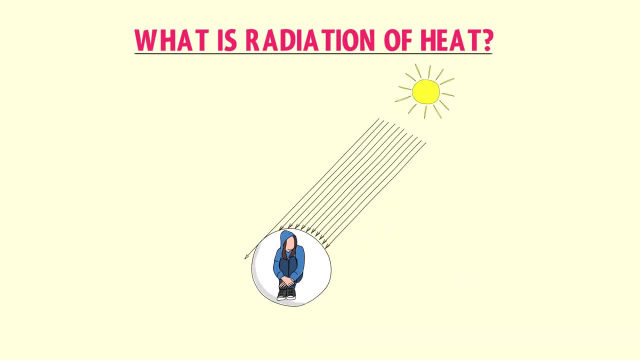 Let consider that during winter days you sit in an open area for the sunlight. Do you feel the hotness of the sunlight? The answer is absolute: yes, We absorb the heat energy of the sunlight. Now here comes the interesting question: Does this heat energy of the sun? 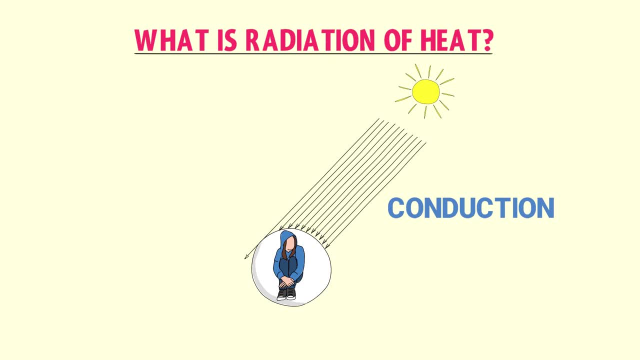 reaches you by the process of conduction of heat? The answer is absolute no, Because there's a large distance between you and the sun. Secondly, does the heat energy of the sun reaches you by the process of convection of heat? The answer is again absolute no, Because when the air absorbs heat energy. 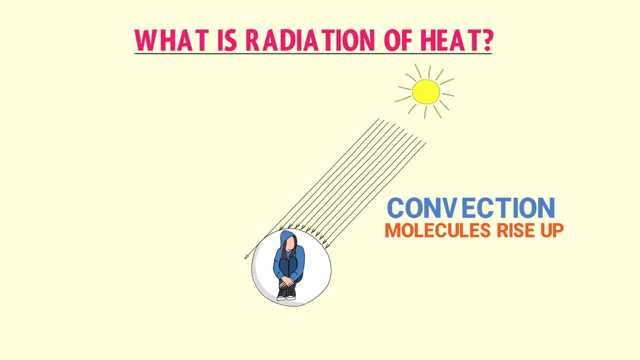 the molecules of air rise up. Secondly, there is vacuum or space between the sun and the earth. Hence the heat energy of the sun doesn't reach you by the process of convection. Then how this heat energy of the sun reaches you? Well, it reaches you by the process of radiation. 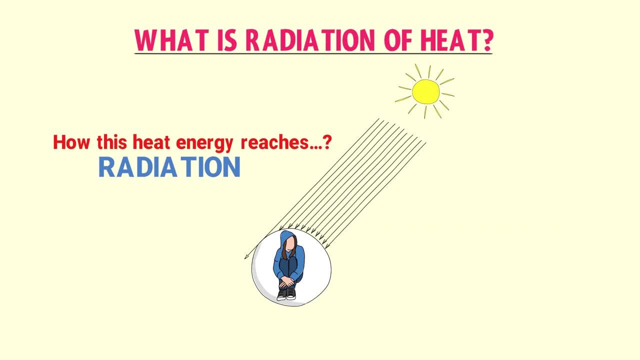 So the heat energy of the sun is transferred by the process of radiation. Remember that radiation of heat doesn't require medium like that of conduction or convection. Thus we can say that the transfer of heat energy without any material medium in the form of radiation,